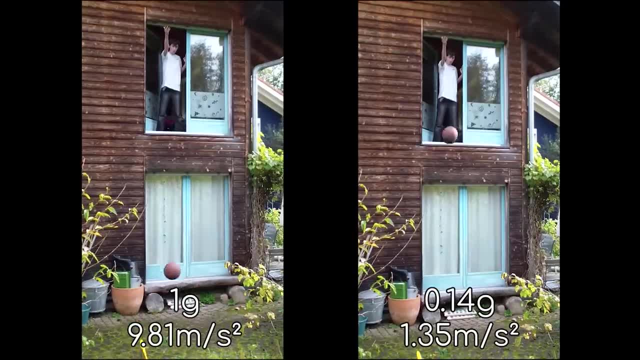 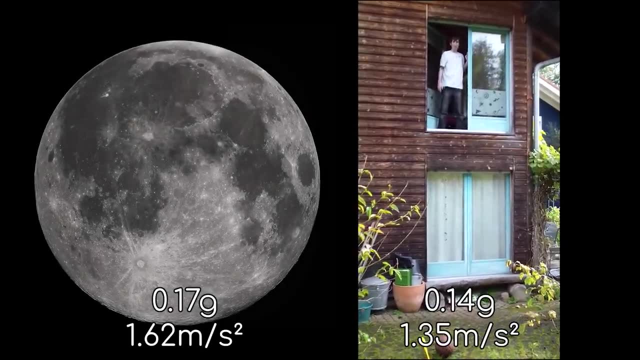 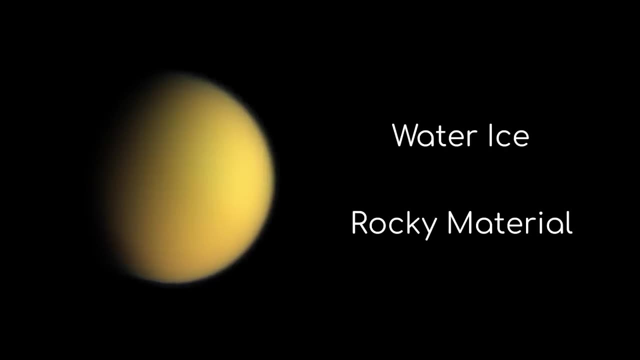 weak at only 0.14 Gs, or 1.35 m per second squared, which is even less than our moon. Due to Titan's low density, it is thought that its composition is half water, ice and half rocky material. Unlike other celestial objects this size, it is believed Titan has. 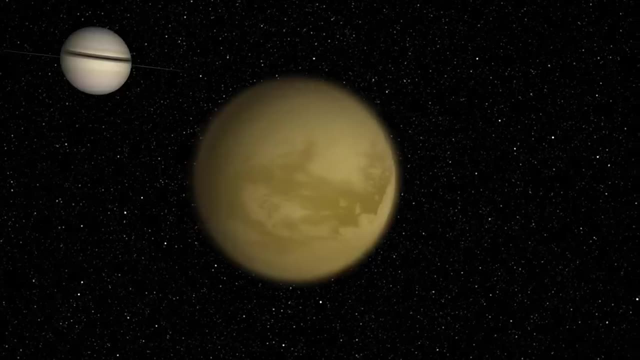 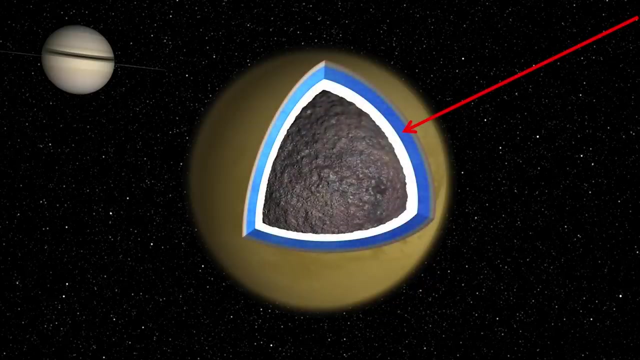 a differentiated interior. This means it has layers, and, like a lot of other large moons, one of those layers is thought to be a liquid ocean comprised of water and ammonia. under the moon's crust, This liquid ocean is comparable to Earth's magma layer, situated between 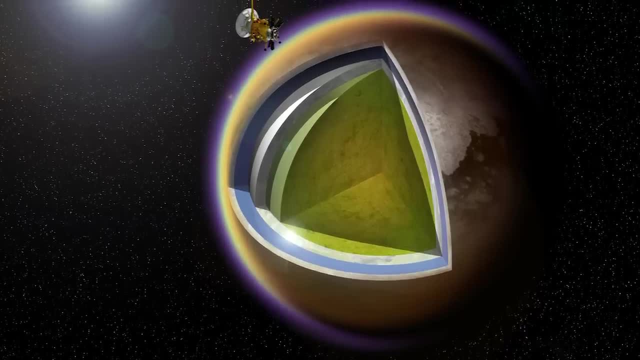 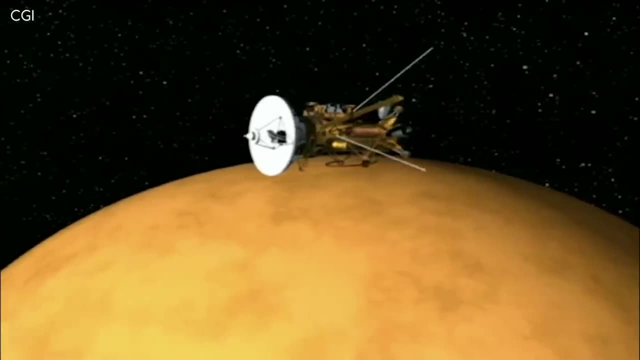 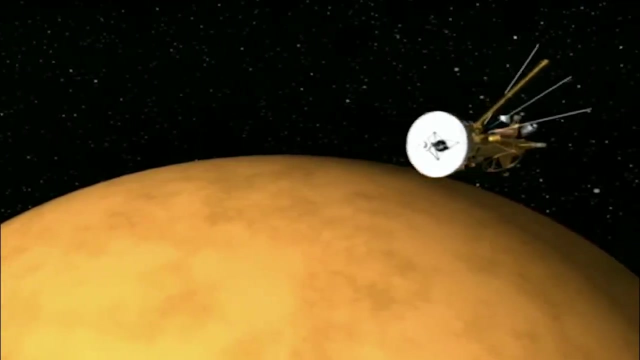 the core and the crust and has been made liquid due to heat pressure and, to a certain degree, tidal forces. The existence of this liquid layer was proven more likely when Cassini, the spacecraft orbiting Saturn, discovered extremely low frequency radio waves in Titan's. 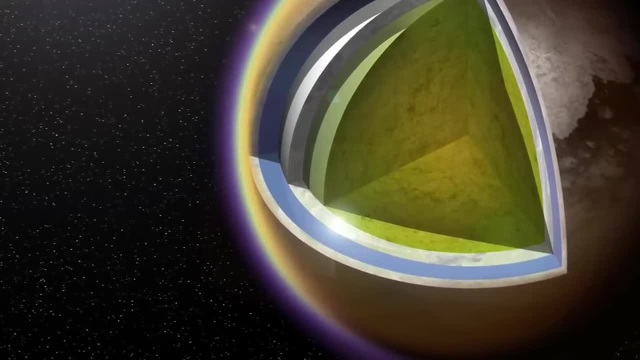 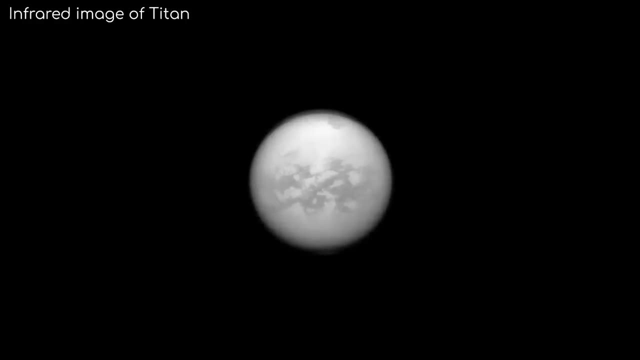 atmosphere. Titan's surface is not known to be a good reflector of low frequency radio waves, but the liquid interior would be. Another reason is that the surface features on the moon have shifted By up to 30km since Cassini started observations, which could imply that the surface is not. 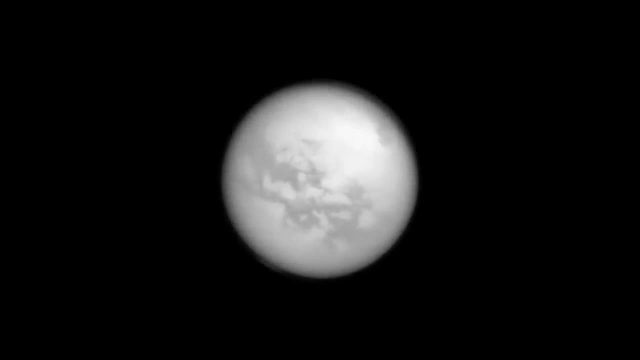 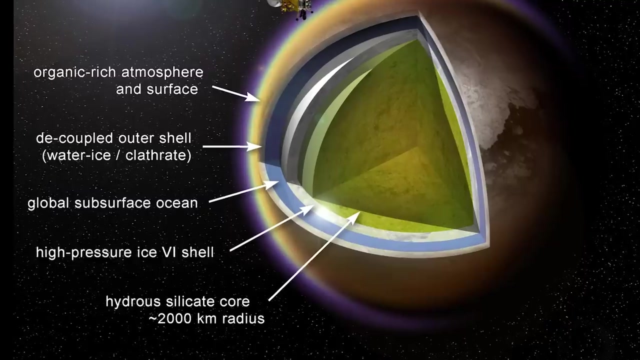 attached to the core, but is rather floating on this liquid ocean layer. And while there is no evidence of life on Titan, scientists do speculate that the conditions would be right for there to be life in this subsurface ocean. Unfortunately, if there was life to 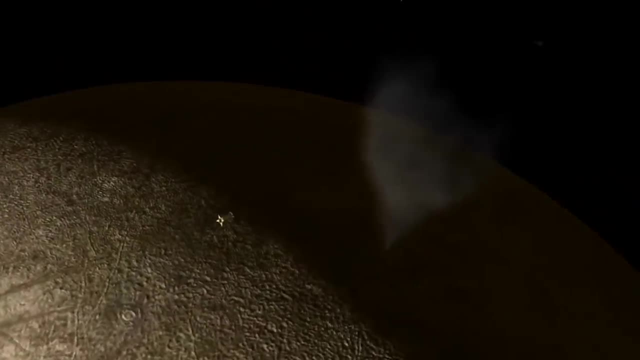 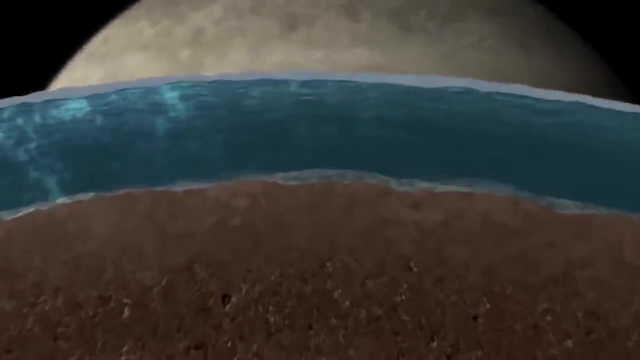 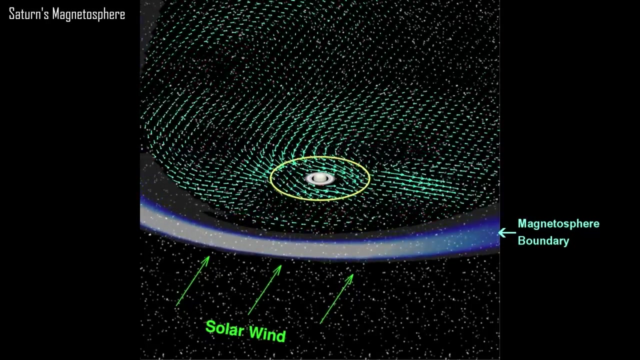 be found on the surface or below. we'll have to wait a while, as there are no planned missions to check out this possibility, And Jupiter's Europa is a more likely candidate to be investigated for life in the foreseeable future. The differentiated interior of Titan does not produce a magnetic field. Titan is still 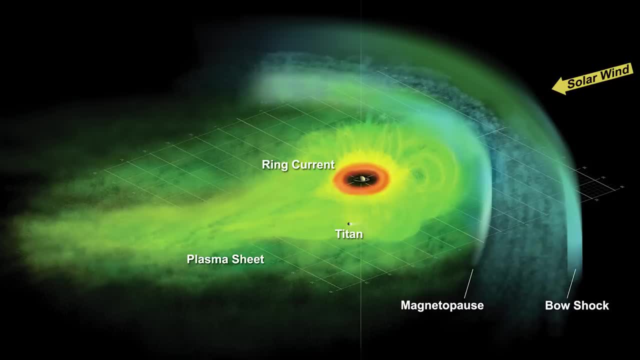 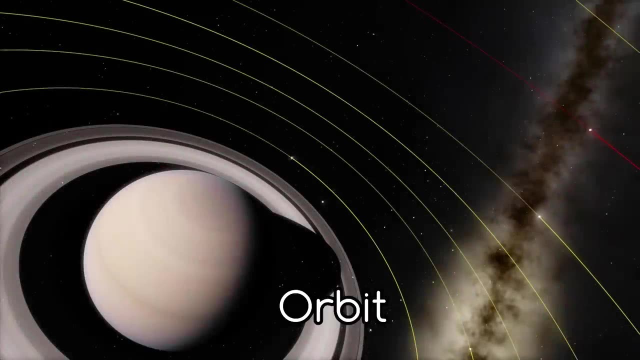 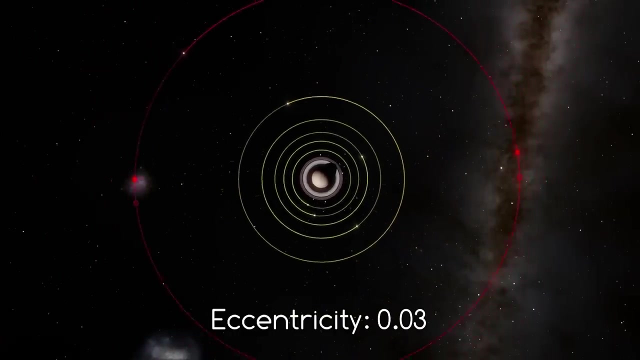 quite protected from the solar wind, though, as 95% of its orbit around Saturn is within Saturn's own magnetosphere. Titan orbits Saturn once every 15 days and 22 hours and has a rather large orbital eccentricity, which means the orbit isn't so large, But what is very interesting is that the orbit 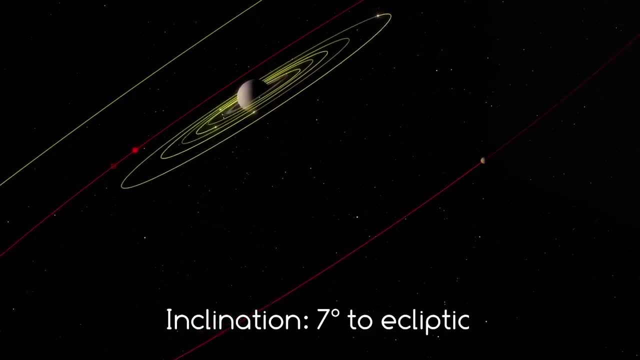 is only 15 days long. So if the orbit of Saturn is smaller than the orbit of Saturn, then the orbit of Saturn would be larger than the orbit of Saturn. and if the orbit of Saturn is circular, Its orbital plane is also at an angle, but that doesn't mean that Titan 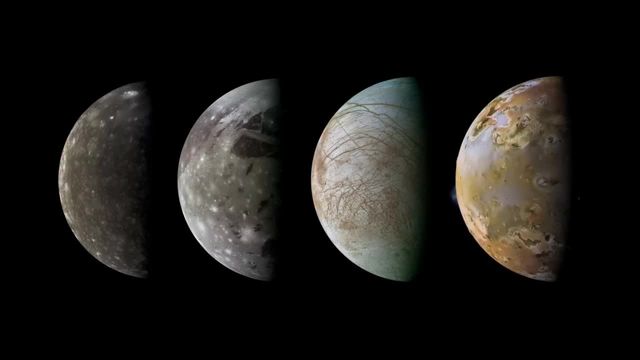 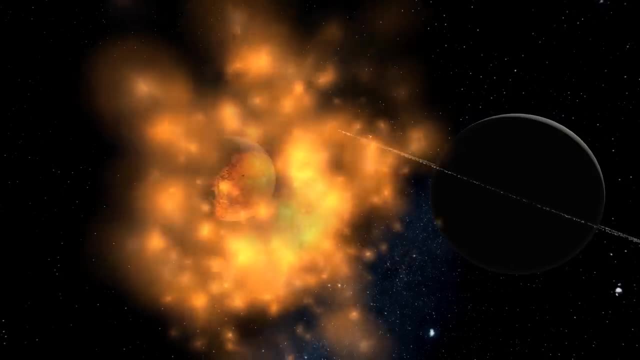 is likely a captured object, Rather like Jupiter's Galilean moons. it is thought that Saturn also had several large moons in the past, but most of these had been destroyed through big collisions, which left Titan the lone victor: Saturn's medium-sized moons. 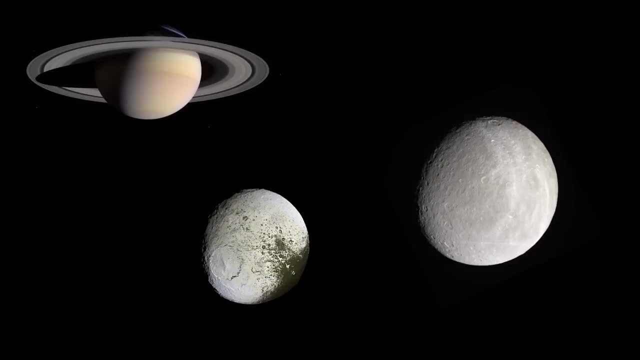 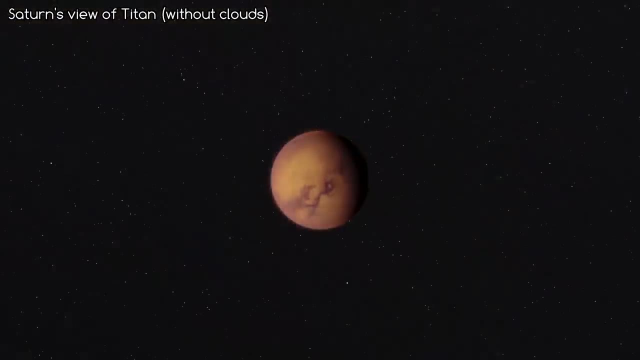 like Iapetus and Rhea, are thought to be the remnants of this tumultuous beginning. Titan's day, like the day on our moon, is identical in length to its orbital period. This means Titan's rotation is tidally locked to Saturn and only ever shows one face to the planet. 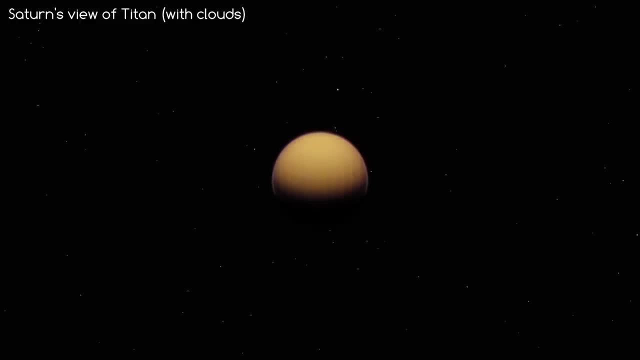 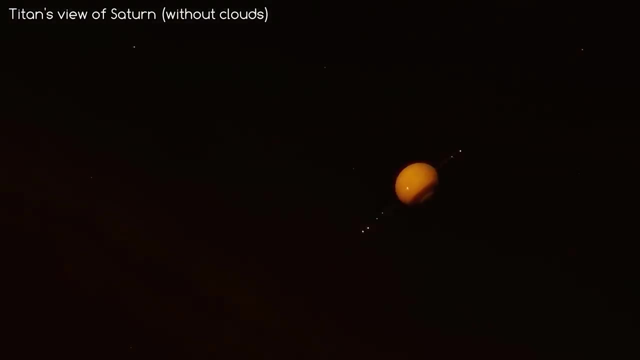 Not that visually it makes any difference. Titan's hazy atmosphere completely blocks the view of the surface from an outside perspective. On the other hand, you might just be able to see Saturn while standing on Titan, although the view would be significantly obscured. 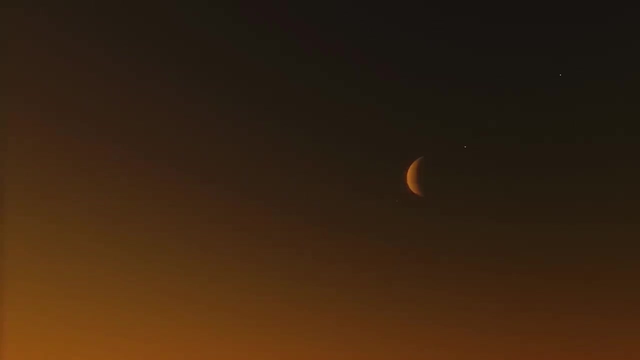 This does mean, however, that if you were to stand on one spot on Titan, you would be able to see Saturn moving. If you were to stand on one spot on Titan, you would be able to see Saturn moving and you'd be able to see the moon move. You'd be able to see. 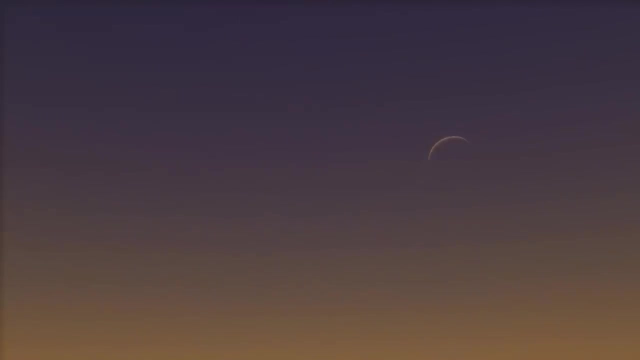 the moon moving, and you'd be able to see the moon move Even if you were to stand on a spot on Titan. Saturn would never move in the sky Removing Titan's haze. this is what it would look like. This leads us on to one of the topics that truly sets Titan apart from the rest of the 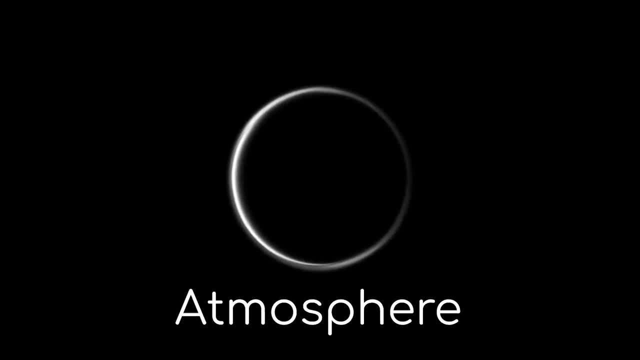 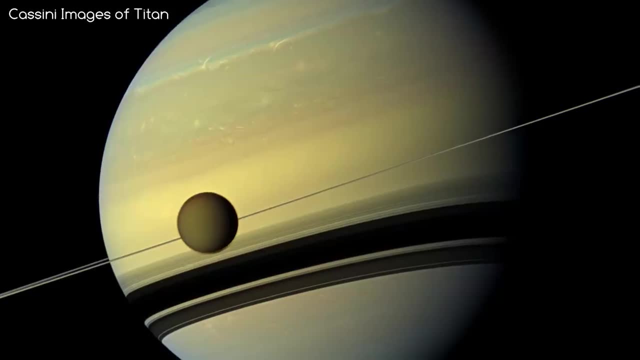 moons in the entire solar system – its substantial atmosphere. I remember the first time I ever saw a photo of Titan. I was truly blown away, as it never occurred to my young self that the moon could even have an atmosphere. I thought to myself. 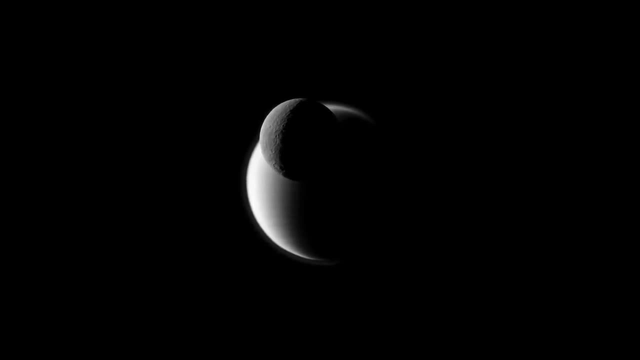 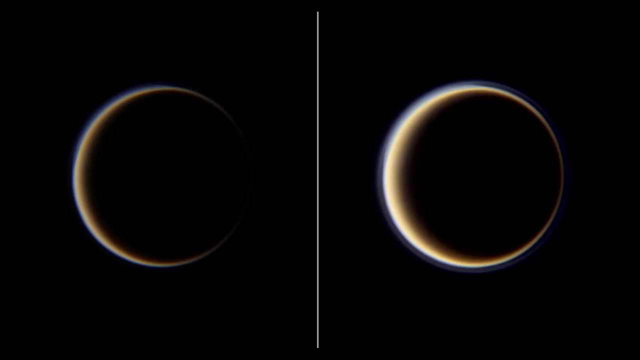 I thought it must have been a new planet they had discovered recently, or something. To me, what looks odd about the atmosphere is how far it stretches into space. When you see a picture of Earth, you see that the atmosphere has quite a tight fit around. 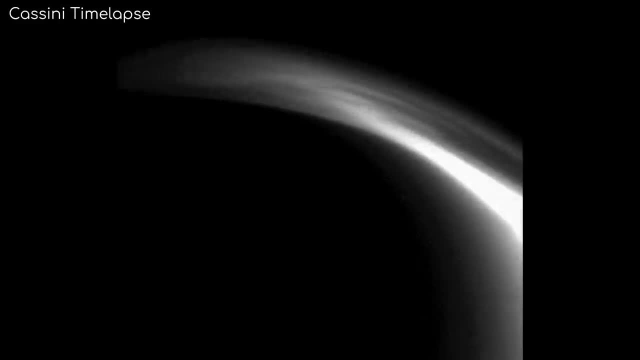 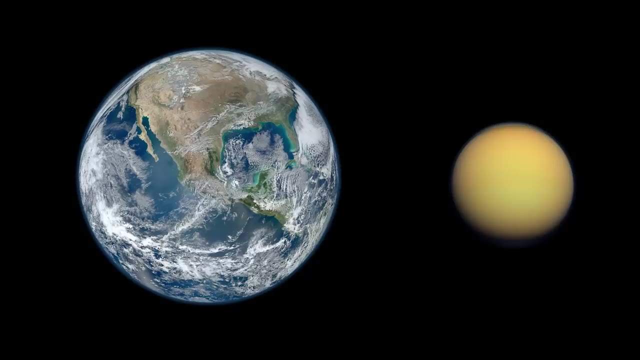 the planet. Titan, on the other hand, looks like it has a thick blanket all over it. There are a number of reasons for this. The first one is that Titan is a lot smaller than Earth, but its atmosphere is 1.9 times. 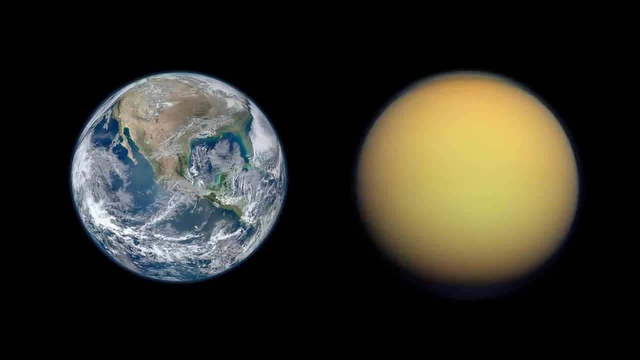 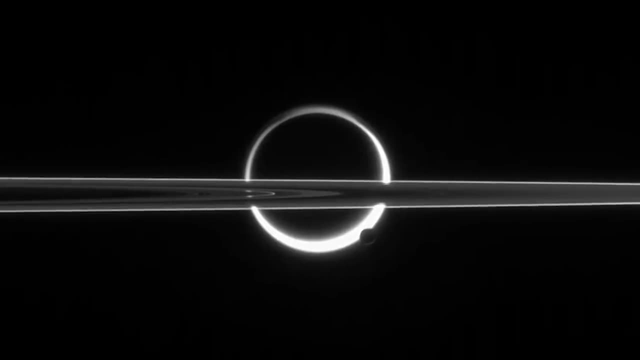 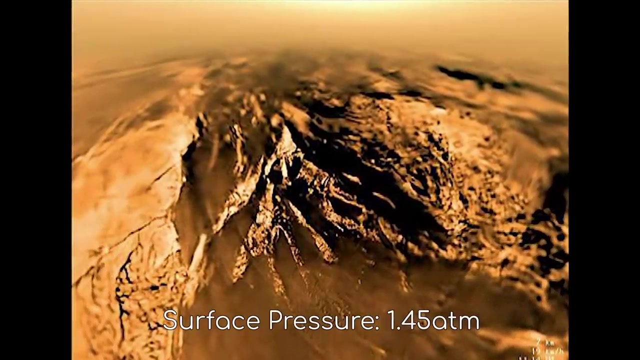 more massive than Earth's, or 7.3 times more massive on a per-surface area basis. The second reason is that Titan's gravity is a lot weaker than Earth's, meaning it doesn't pull it down as strongly. The mass of the atmosphere actually means the pressure at the surface is 1.45 atmospheres. 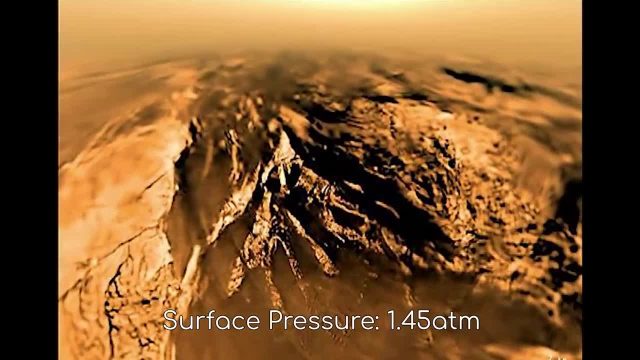 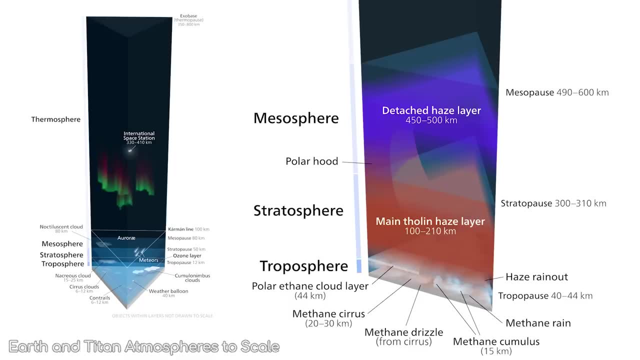 or 45% more than the atmospheric surface pressure on Earth, And comparing the two you can see the extent of how far Titan's atmosphere stretches into space. 600km high is only the limit of the mesosphere. Earth's mesosphere, on the other hand, stops at 120km. 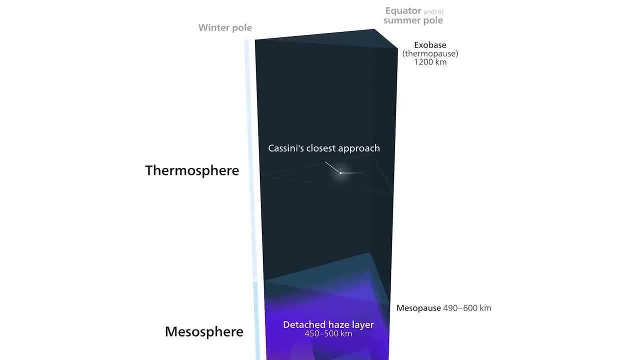 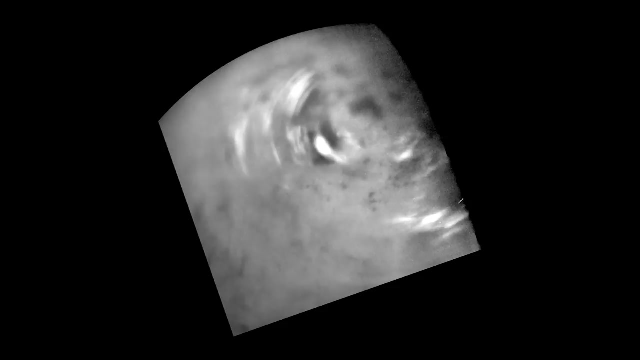 Even at a distance of 975km, the Cassini spacecraft had to make adjustments to maintain a stable orbit against atmospheric drag when it made its closest approach. Like Venus, Titan is a super-rotator, meaning its atmosphere rotates faster than the rotation of the planet. 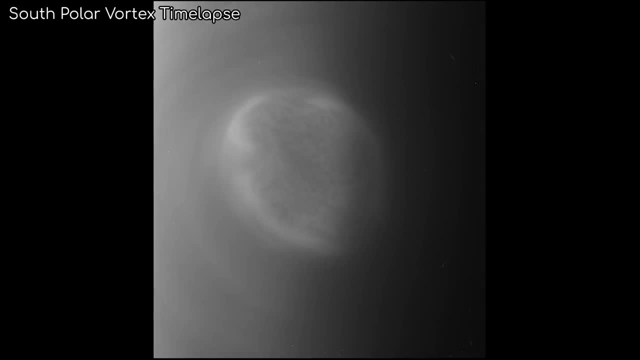 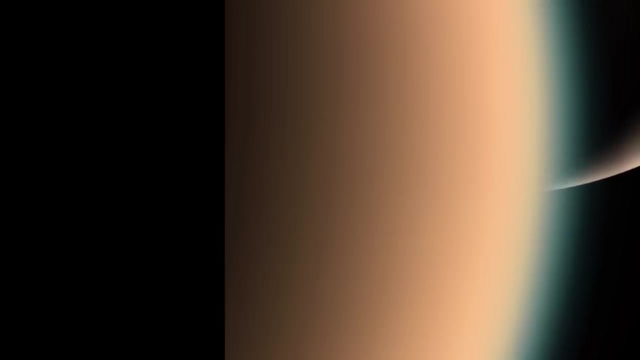 This can especially be seen at the poles on the Moon. Each pole has a polar vortex that rotates once every 9 hours, compared to the Moon's rotation of 16 days. The vortexes on each pole seem to be like permanent hurricanes. So what does the atmosphere consist of, and why is it orange in colour? Well, the atmosphere is 98.4% nitrogen, the remainder being mainly methane and a small amount of hydrogen. There are also trace amounts of hydrocarbons from the breakup of methane in the upper atmosphere due to UV light, And it is these hydrocarbons that are thought to give Titan its orange hue. 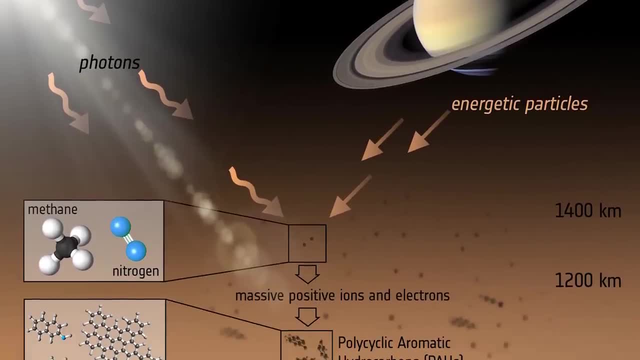 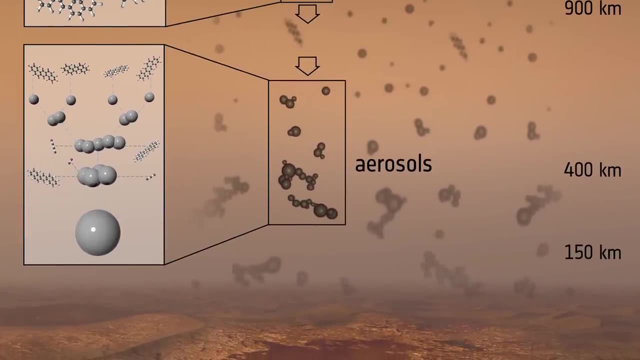 This constant breakup of methane to hydrocarbons should have meant the Moon ran out of methane within 50 million years, a very short space of time compared to the age of the solar system. This means that there must be a source that replenishes the methane, though most likely. 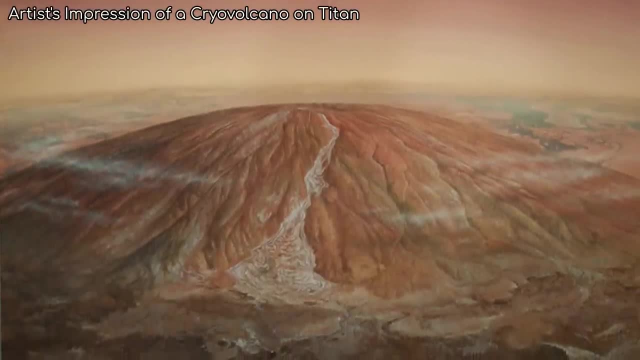 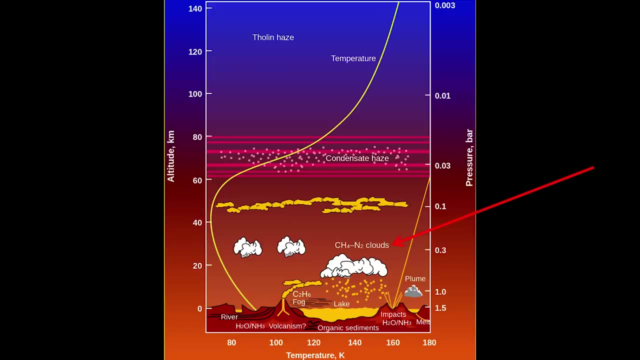 candidate being cryovolcanoes, although biological life has not been ruled out. The methane in the atmosphere creates a greenhouse effect, without which the temperature on Titan would be a lot lower. Conversely, however, the haze also reflects a lot of the sunlight, creating an anti-greenhouse effect which cancels out some. 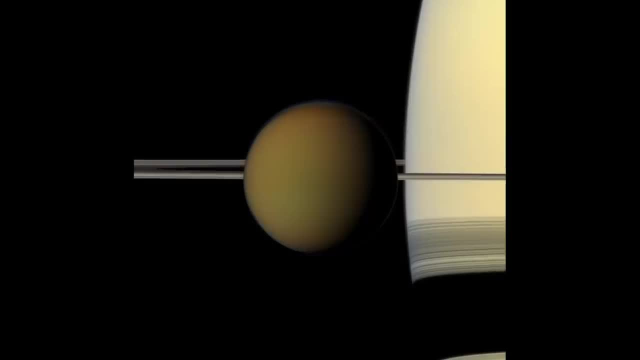 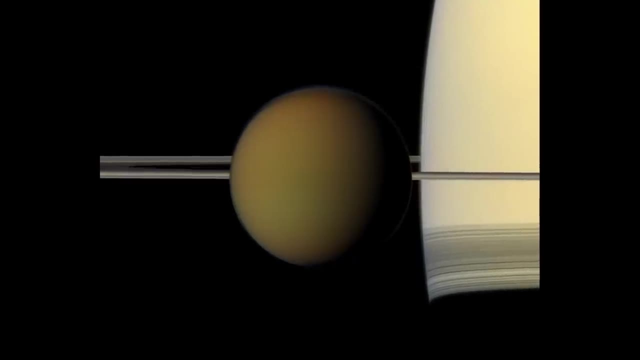 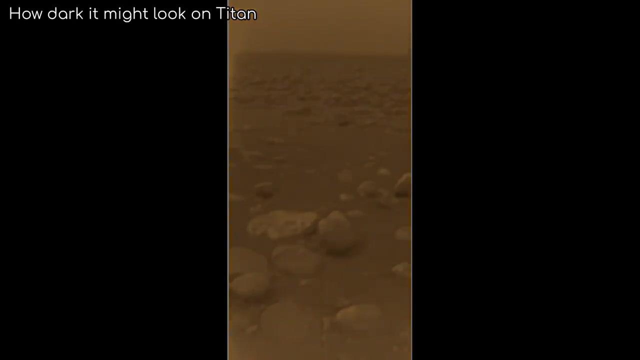 of the potential greenhouse effect from the methane. Now, while Titan's upper atmosphere gets 1% of the sunlight, Earth does, due to the distance from Titan to the Sun, another result of this reflection of sunlight means the surface of Titan only gets about 0.1%. in the end, The 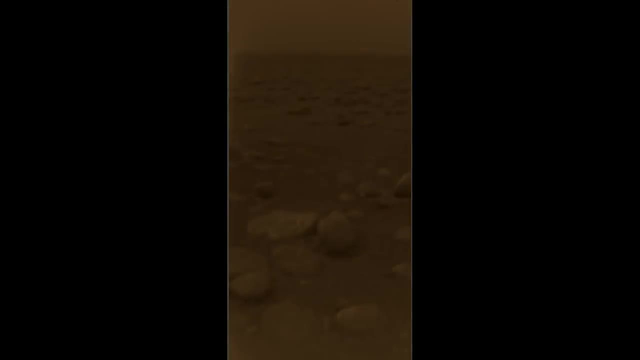 Huygens team liken the difficulty of taking photos at this light level to taking pictures of an asphalt parking lot at dusk. All these things combined means that, while it would be dark, a human would only need an oxygen mask and, to wrap up, extremely warm. 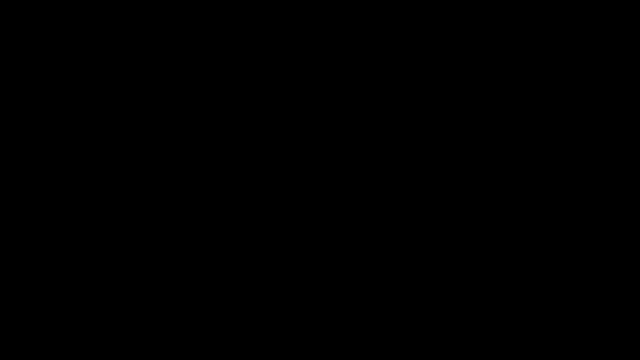 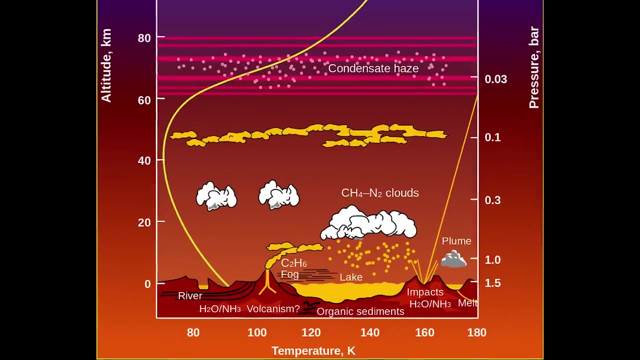 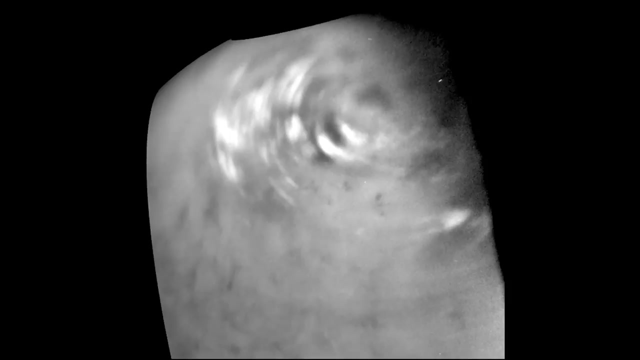 be comfortable while standing on the surface of Titan. It really is cold on Titan: minus 180 degrees centigrade on average. This means any water on Titan remains solid and doesn't ever melt, evaporate or sublime. Then why are there sometimes clouds on Titan? Well, these are not water ice clouds, but rather methane clouds, which means, yes, it can rain methane on Titan. The temperature on Titan is just right for methane to be liquid. Methane freezes at minus 182.5 degrees centigrade and boils at minus 161.5 degrees centigrade The temperature. 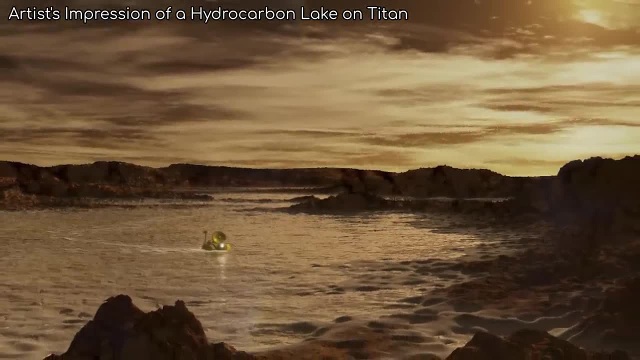 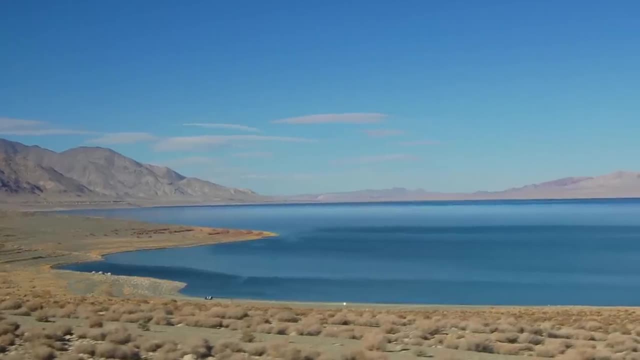 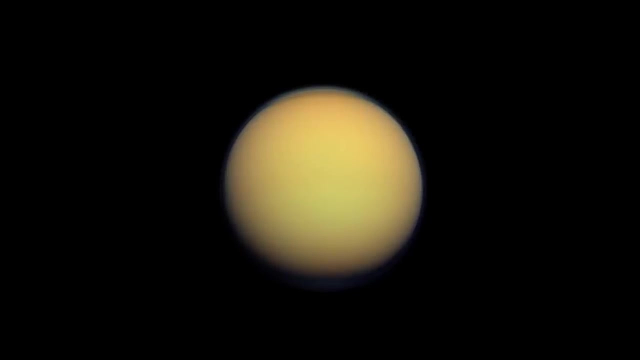 combined with the surface pressure, got scientists very excited at the prospect of there being hydrocarbon lakes, or seas on the surface of Titan, similar to water lakes and seas on Earth. If there were really lakes on this moon, it would be the first time this had ever been observed outside of Earth. 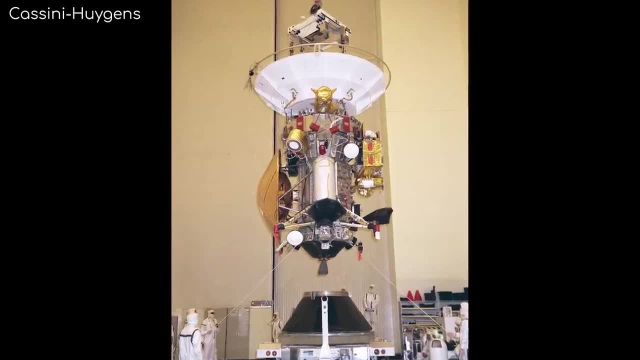 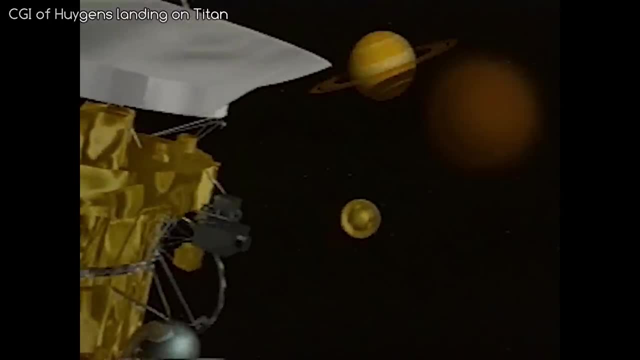 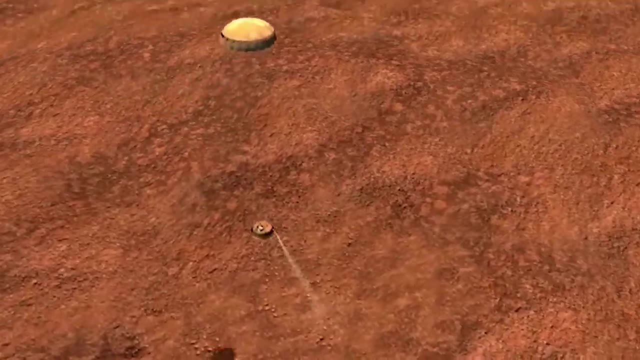 This was actually one of the main driving forces behind Cassini-Huygens: to see what there was under that thick atmosphere. The Huygens probe, named after the astronomer who discovered Titan in 1655, was designed to enter Titan's atmosphere and land on the surface. 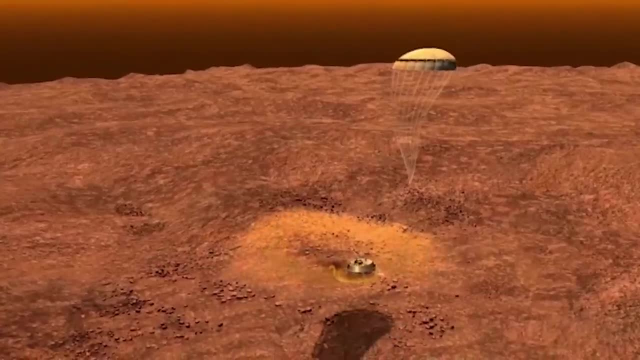 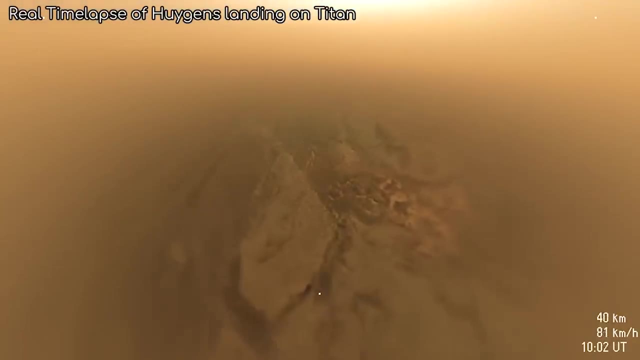 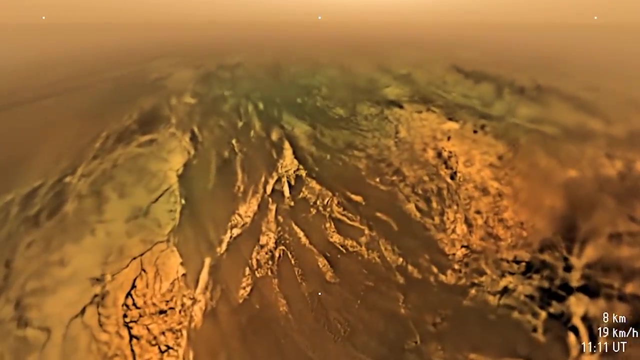 The possibility of even landing on an ocean was taken into account during its design process. As the probe descended, its parachute was pulled and after an almost three-hour journey, it finally rested on the solid surface of Titan. Sadly, it wasn't able to see any lakes, but what it did see confirmed that methane. 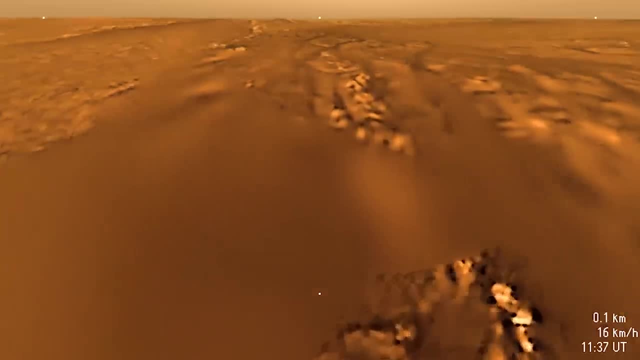 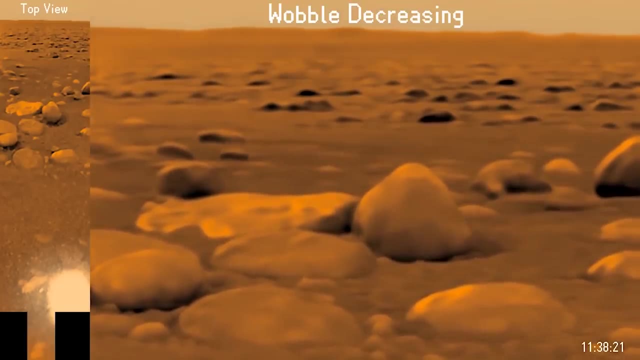 lakes once existed. as Huygens landed on what appeared to be a dried-up lake bed, The stones you see from the surface photos are rounded stones, much like pebbles found in a river or a lake on Earth. Cassini from the perspective of space. 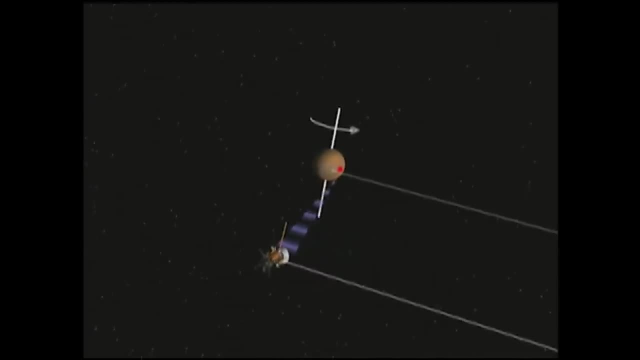 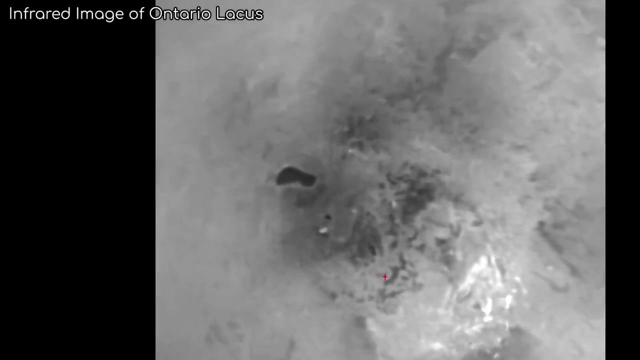 was able to confirm that methane lakes are still found on Titan today. Near the South Pole, Cassini observed an area which was later confirmed to be a lake called Ontario Lacus. It is 20% smaller than its North American namesake, Lake Ontario. 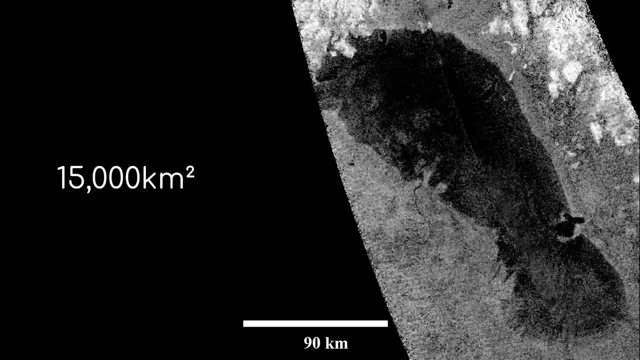 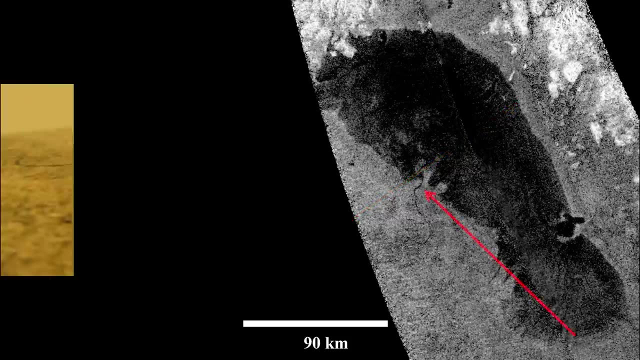 So in other words, it is still pretty big at 15,000 square kilometres. On this side of the lake you can see a smooth shoreline eroded by waves. On the west side you can see the first evidence of a river. 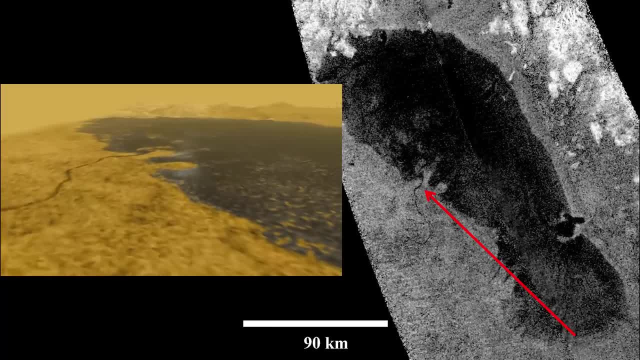 Cassini, from the perspective of space, was able to confirm that methane lakes are still found on Titan today. The second evidence was that methane lakes were found on Titan, meaning that liquid hydrocarbons flow down higher plains to the lake, leaving delta deposits in much the same process. you 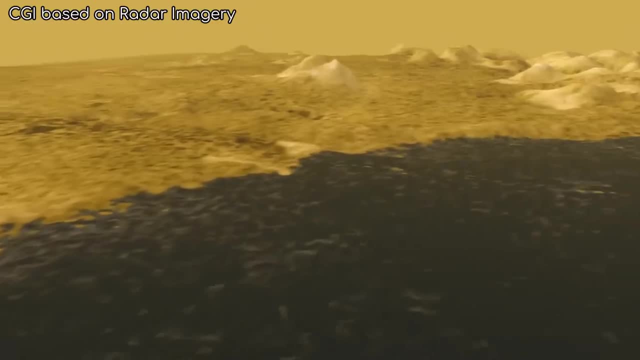 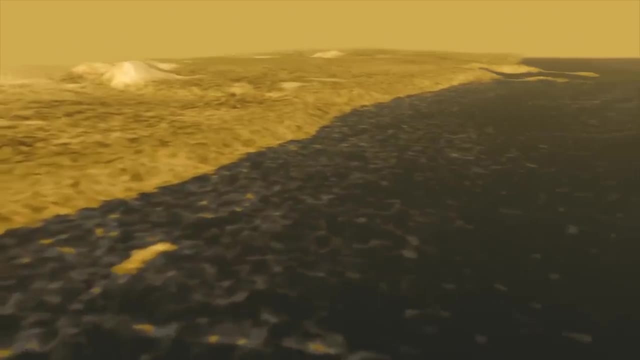 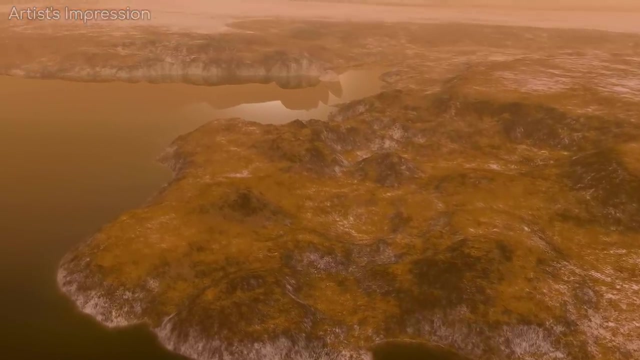 would find on Earth. Ontario Lacus is extremely shallow, only estimated to be between 40 cm and 3 metres deep, the deepest point likely to be just over 7 metres. As Cassini's radar mapped this lake, it found that the lake did not have waves bigger than. 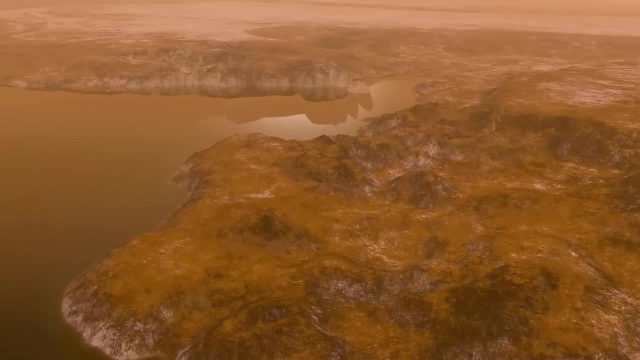 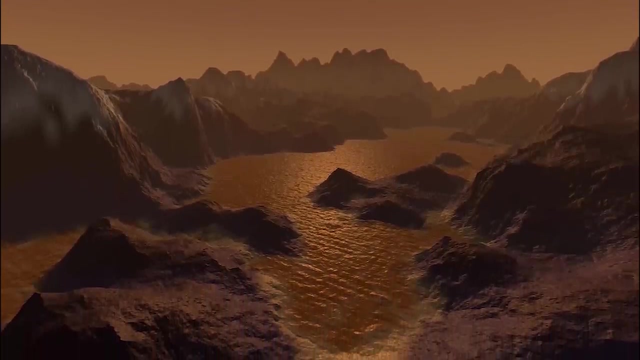 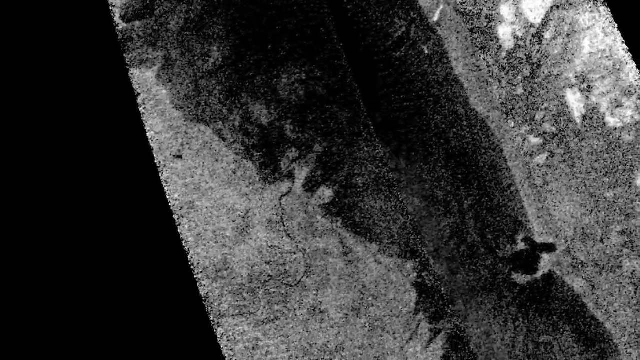 3 mm, the surface would appear like a sheet of glass or a mirror. This doesn't mean there can't be bigger waves, unless this liquid is particularly viscous, but the likelihood is that it was simply not a windy day as the observations were taken. The atmospheric density and gravity 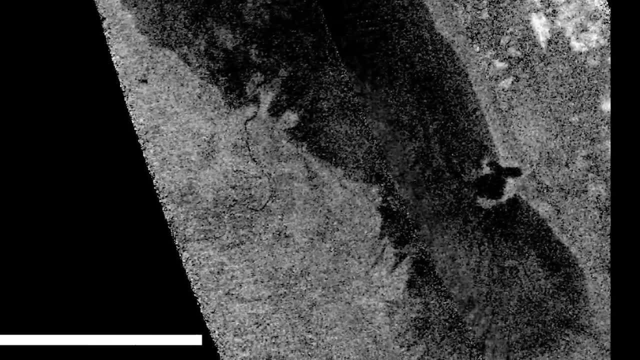 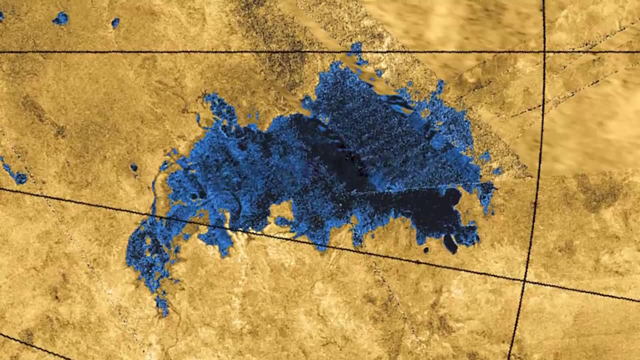 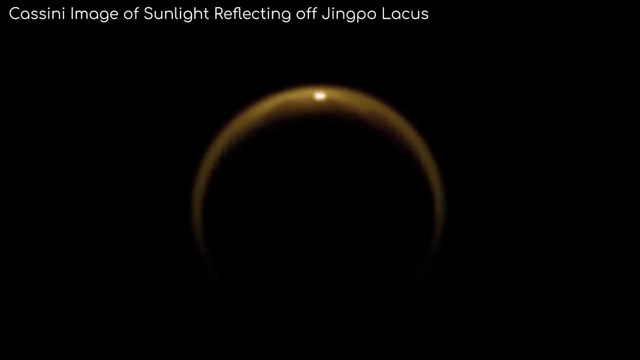 on Titan should mean that waves would be bigger on Titan than they would be on Earth. As the north pole of the moon began to come out of a 15 year winter, another lake was discovered, Jingpo Lacus. As Cassini was passing by the moon, sunlight was reflected. 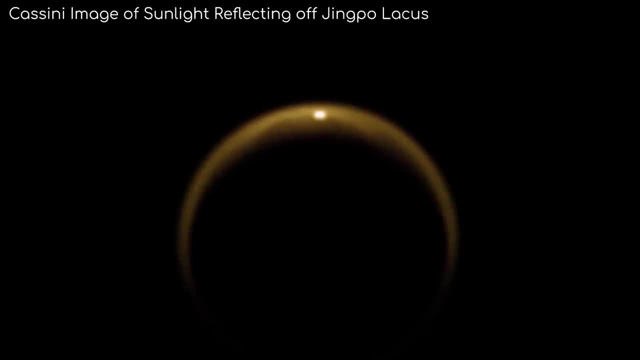 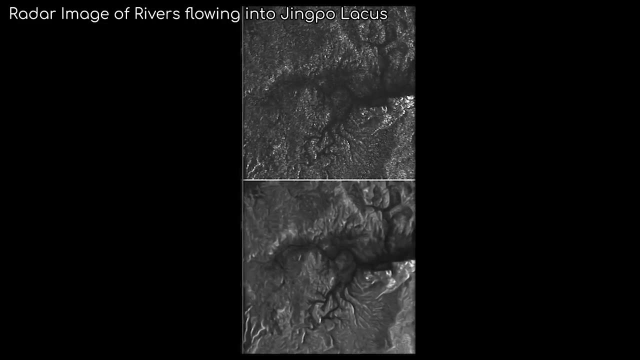 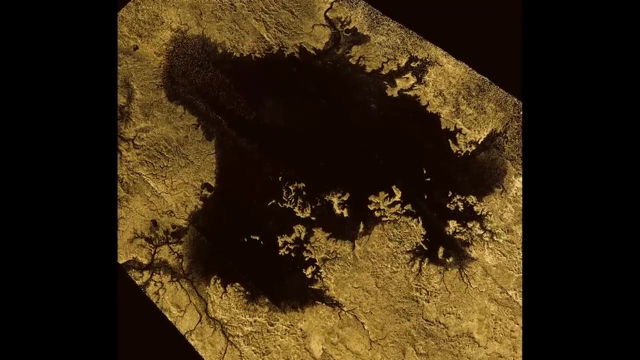 off the surface of Jingpo Lacus like a mirror, directly into the view of Cassini. Upon further observation, Cassini was able to detect further evidence of moving liquid on Titan, as can be seen by these rivers flowing into the lake. The second biggest lake on Titan to be discovered is Ligia Mare, found in the north polar region. of Titan. It is bigger than Lake Superior on Earth, with a surface area of 126,000 square kilometres. While parts of this lake are reasonably shallow, the average depth is a lot deeper than Ontario Lacus, at 50 metres, and some parts of it could reach depths of over 200 metres. Plenty of 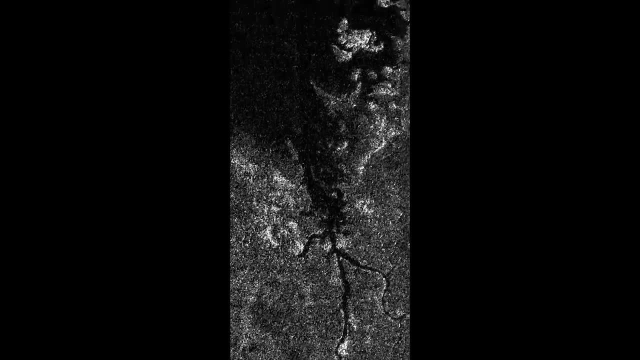 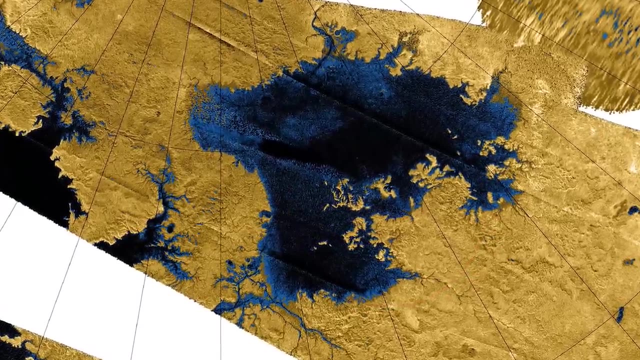 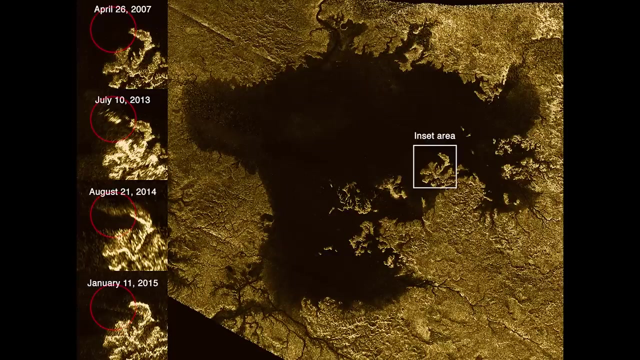 rivers can be seen flowing into the lake, and there are large islands found around this area. here A particularly curious observation Cassini made- The largest lake on Titan, dubbed the Magic Island, is the appearance and disappearance of what appears to be an island, Although scientists are unsure exactly what happened. 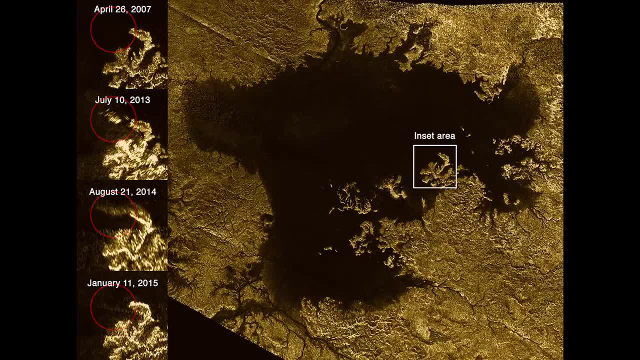 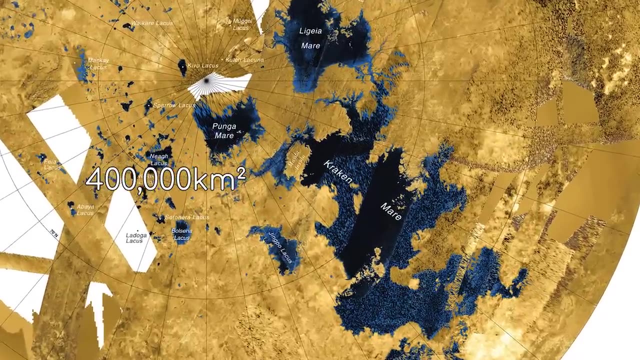 here. the theories are that it could be silt suspended in the lake bubbles or subsurface ice rising to the surface as the lake warmed during the moon's spring. But still very curious. The largest lake on Titan, at 400,000 square kilometres, is the Kraken Mare, The largest 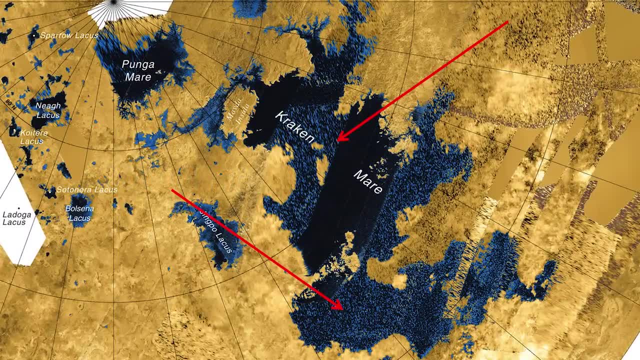 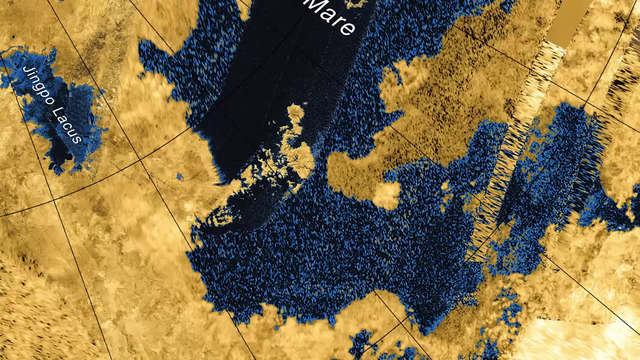 lake on Titan at 400,000 square kilometres, is the Kraken Mare. As you can see, the lake is split up into two main parts, separated by a small stretch quite similar to Earth's Strait of Gibraltar. Its nickname is the Throat of the Kraken. 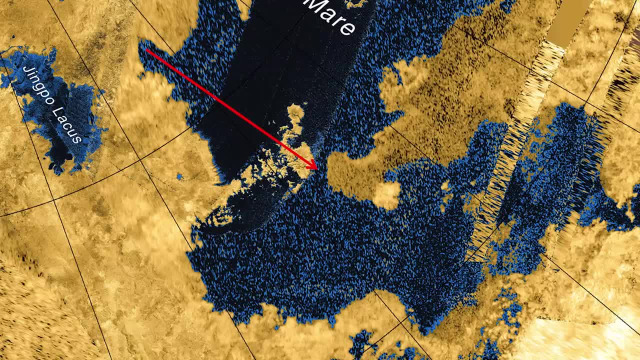 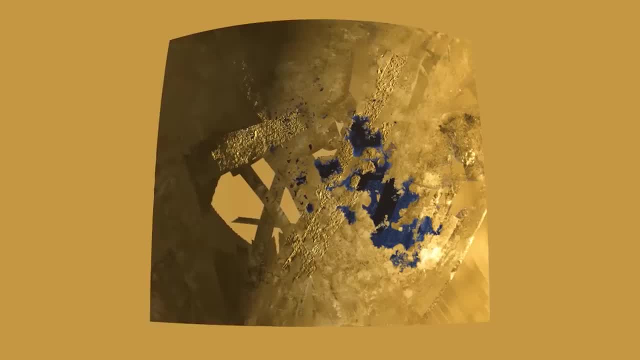 Because of tidal forces and the size of the lake. it's thought the tide changes by about 1 metre, and so this strait may have strong currents and even whirlpools. The Kraken Mare is also quite deep in comparison to Ontario Lacus, but isn't any deeper than 170 metres. 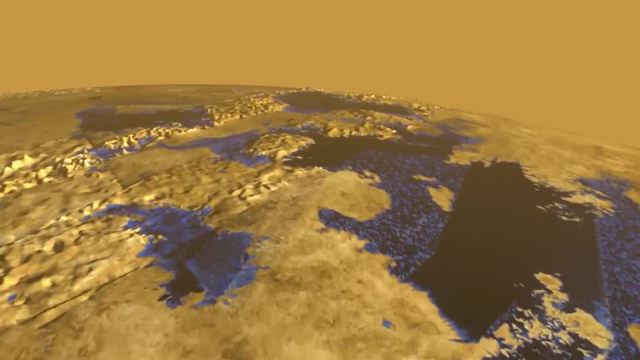 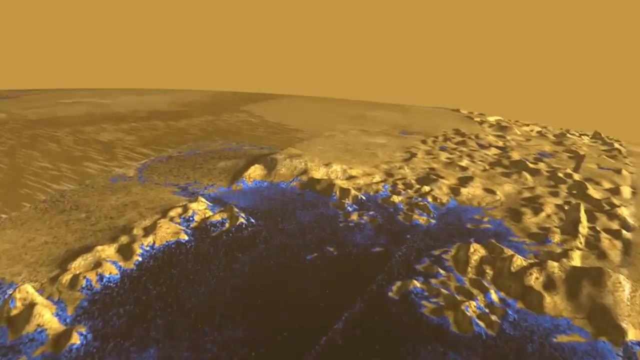 The Kraken Mare is also quite deep in comparison to Ontario Lacus, but isn't any deeper than 170 metres. So we know about the lakes on Titan now, but what other interesting surface features might it have? Well, plenty actually. Titan's surface is quite young, as young as 100 million. 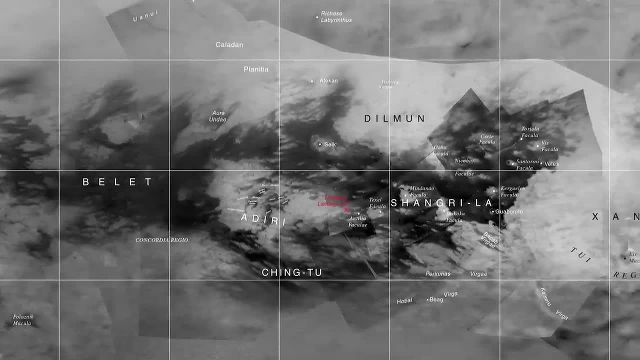 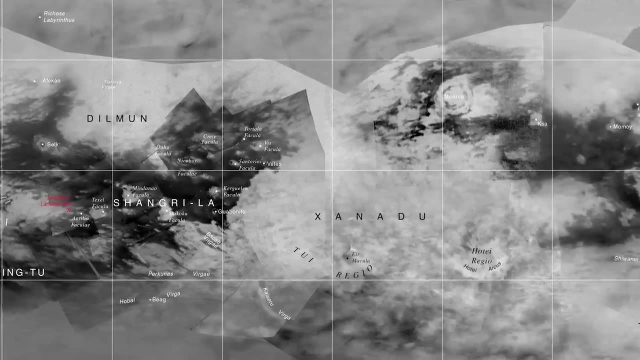 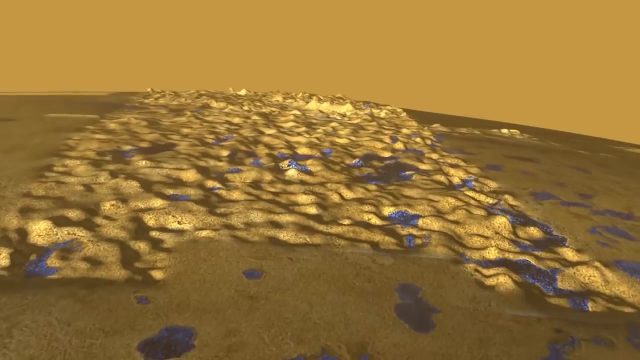 years old, which means its surface must be geologically active. Some scientists believe the dirty ice crust is substantially rigid, although there is some evidence to suggest that there is tectonic activity on the moon, possibly caused by tidal forces with certain factors. The main factor of a renewed surface, however, is likely to be the same thing: that 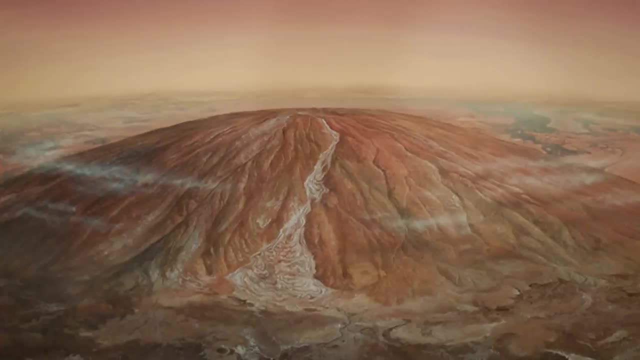 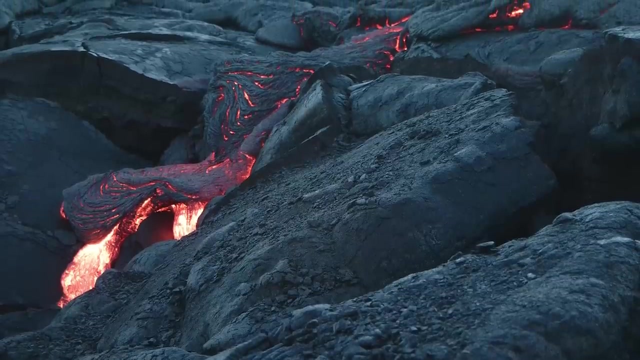 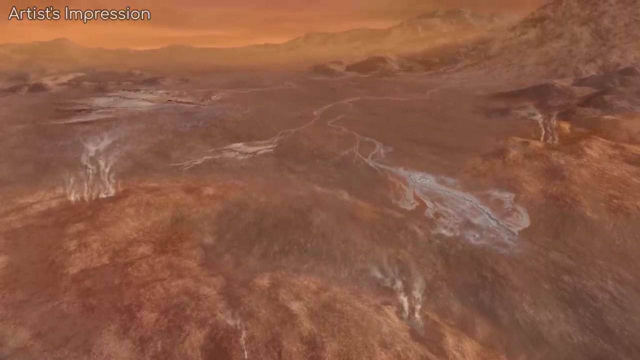 produces methane in the atmosphere – cryovolcanoes. Now, this is pretty interesting. You know how magma on Earth is pretty hot, But when it comes out of the ground it freezes. Well, Titan has the same thing, except its magma is water and ammonia, and when it comes out, 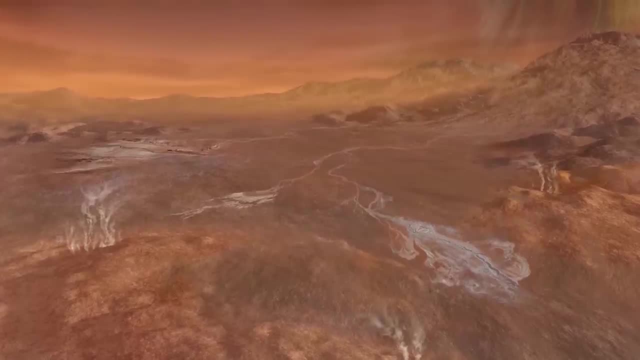 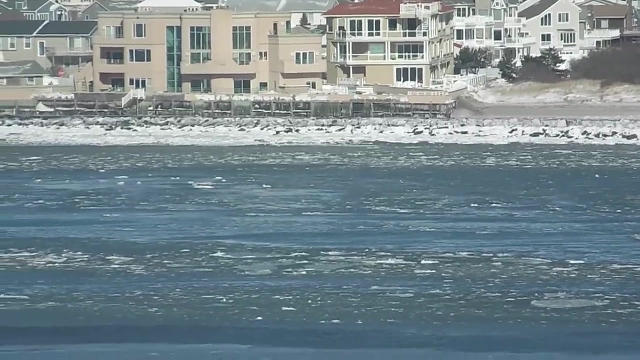 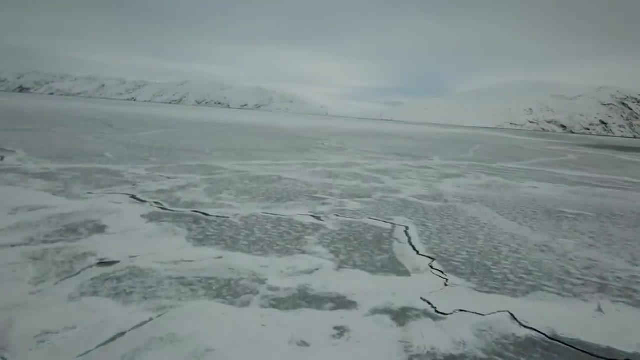 of the cryovolcanoes and spills over the land, it too freezes to renew the surface. Because a water and ammonia blend is a lot less viscous than lava. it flows further than lava on Earth. This means mountains are more flat and will never reach the heights of volcanoes on Earth. 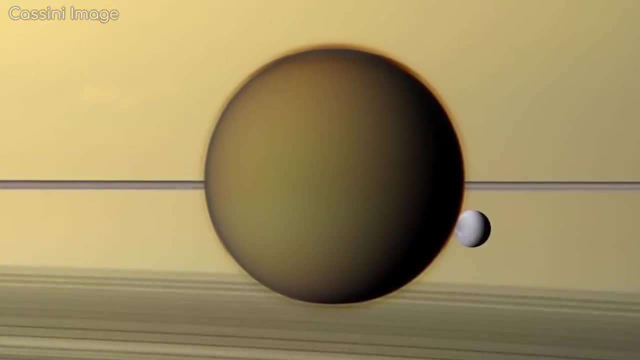 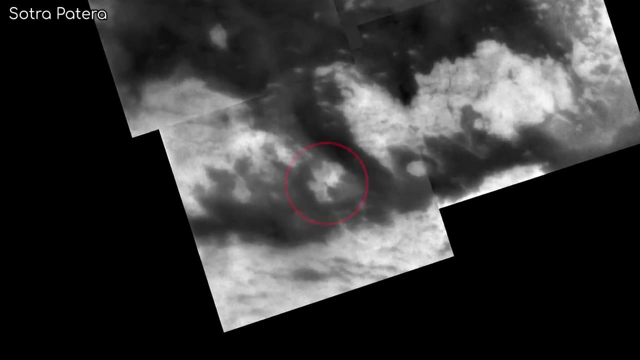 While it is hard to confirm specific cryovolcanoes on Titan due to the obstruction caused by the atmosphere, the most likely candidate is Sotra Patera, found on the southern hemisphere. In this image, height has been exaggerated by a factor of 10,, but it gives a good idea. 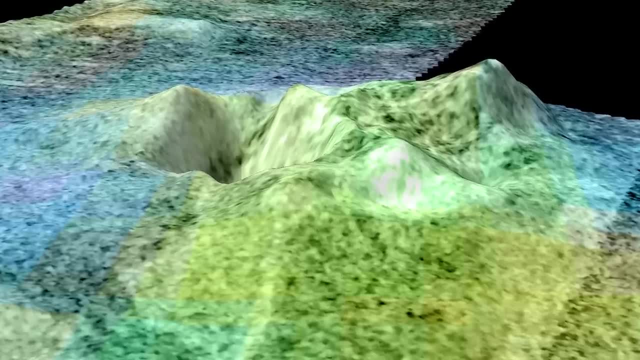 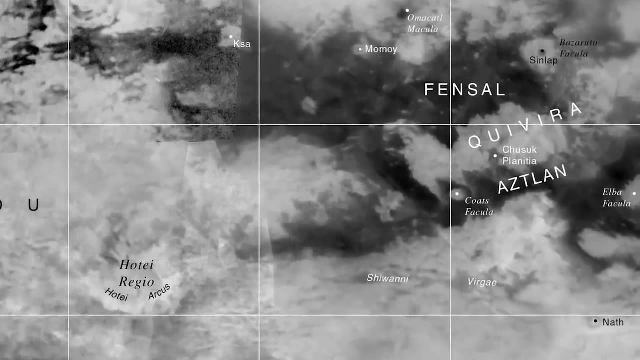 of the surface. Sotra Patera is one of the highest-growing volcanoes in the world and it is the largest that we know of on Titan. The force necessary for this to erupt would have had to have been incredible, and while it doesn't appear to be active now, it is being actively monitored. 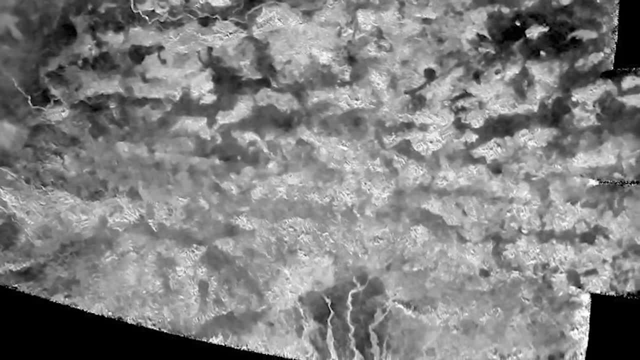 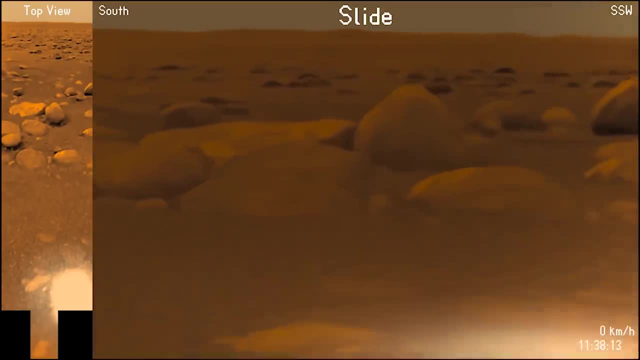 The fact that lava on Titan is a mix of water and other minerals means the surface could be compared to dirty ice, Because we know the Huygens bounced and wobbled in a certain way as it landed on Titan. we have a rough estimate of the surface. 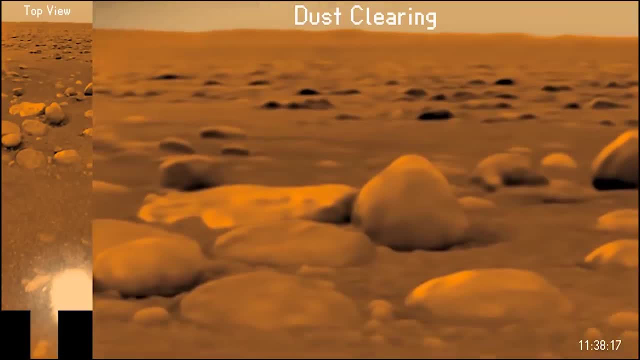 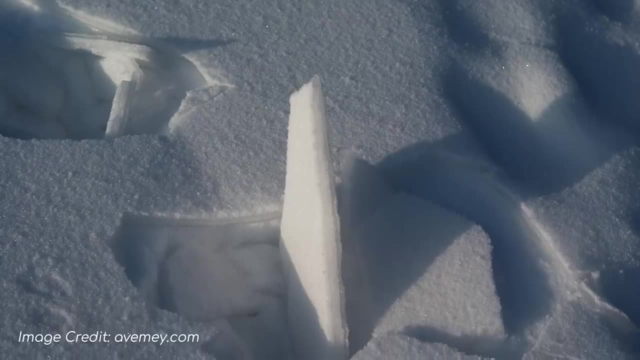 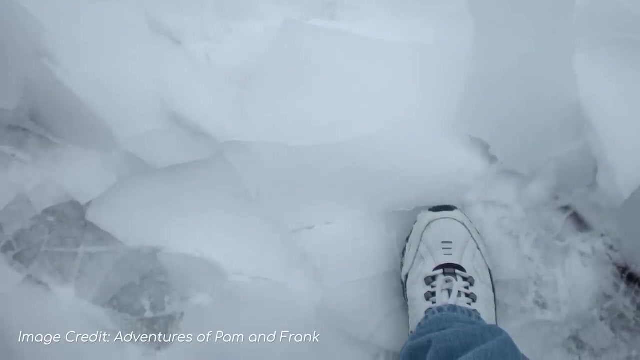 Scientists have referred to it as a soft, damp sand. Another theory is that it's like snow with a thin crust on top. Imagine walking on frozen snow. If you're careful, you can walk on a solid surface, but if you stomp too hard you will sink in quite deeply and 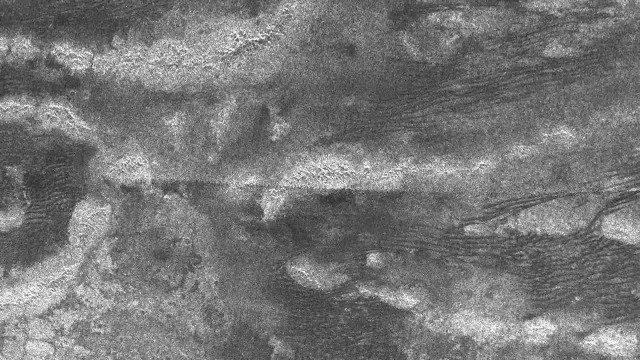 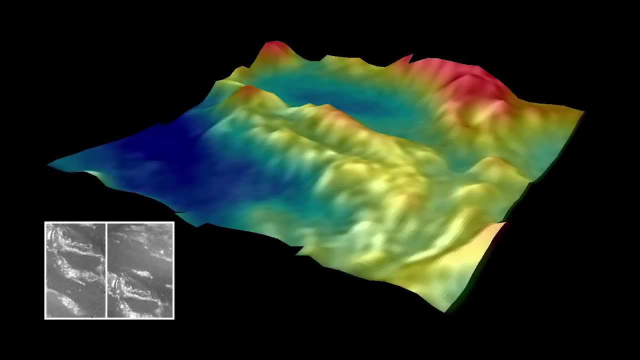 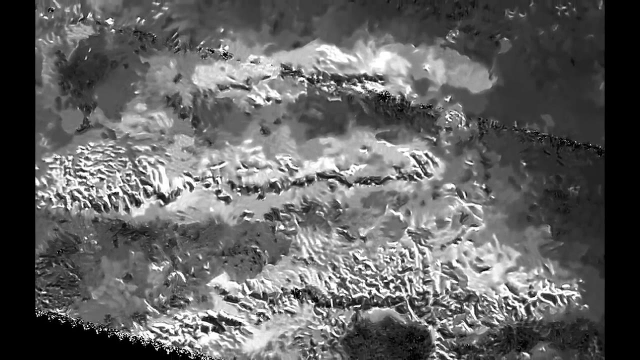 Titan is believed to be something like this. Titan's highest mountains come in the form of ridge belts, like the Rockies in a mountainous city in America. These ridge belts could also be a form of cryovolcanoes. The largest mountain on Titan can be found in one of these mountain ranges, known as Mithrim Monts. 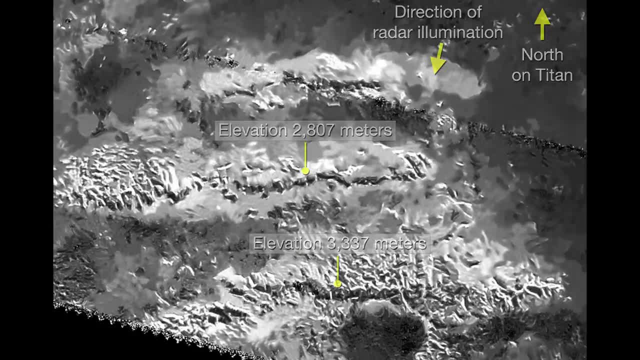 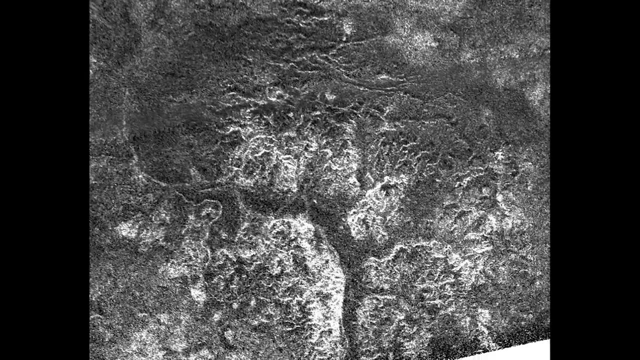 and is 3,337 metres high. Interestingly, mountains this tall are thought to be topped with methane snow. Also found on Titan are many gorges, valleys and dunes. Using infrared cameras to see the surface from space, they can be found on Titan. The largest mountain on Titan can be found in one of these mountain ranges known as Mithrim Monts. Also found on Titan are many gorges, valleys and dunes. These gorges can be found in one of these mountain ranges known as Mithrim Monts. Also found on Titan are many. 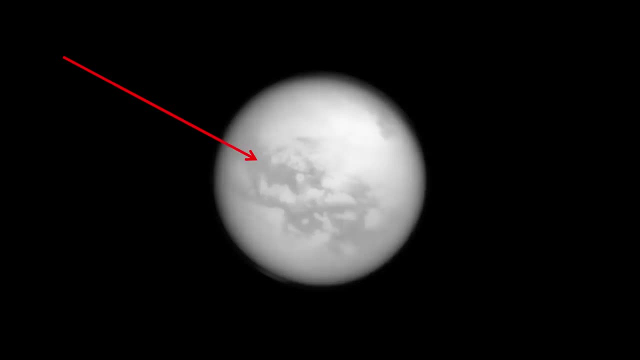 gorges, valleys and dunes. Using infrared cameras to see the surface from space, they can be found. on Titan are many gorges, valleys and dunes. What can also be seen quite prominently are these large patches of dark terrain. Originally, these dark patches were thought to be seas until the Huygens probe landed. 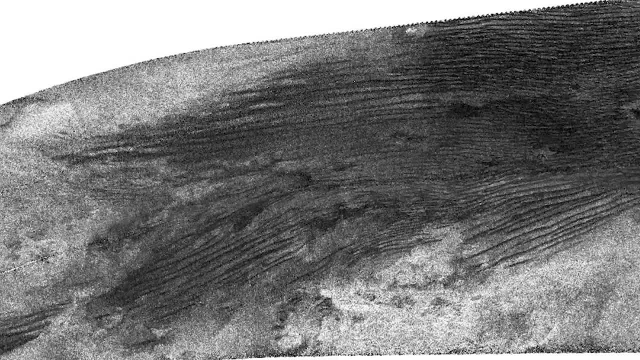 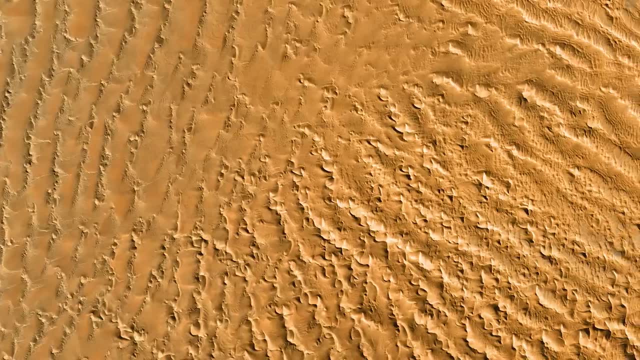 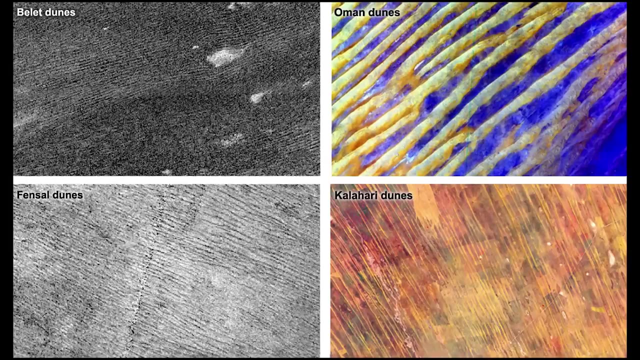 on one of those areas known as Shangri-La. They could well have been seas in the past, but now they are plains of dark mineral deposits, similar to the Namib Desert on Earth, where they appear as windswept dunes in some places. 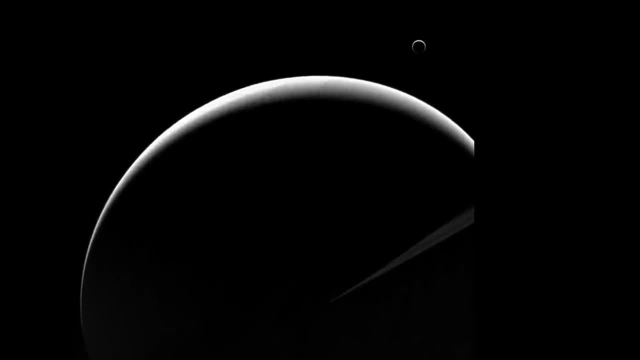 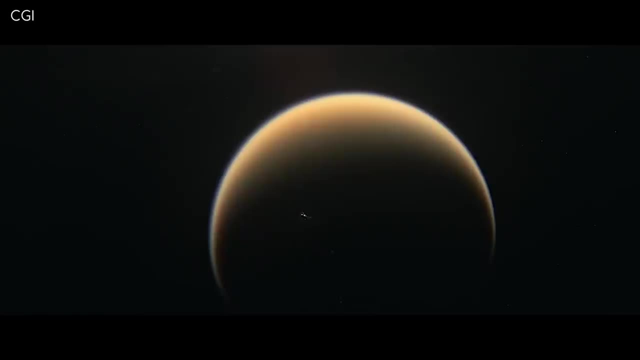 Overall, Titan can be compared to Earth in lots of ways. Scientists think that Titan shows signs of what early Earth could have been like, only much colder. It's fair to say that Titan is remarkably interesting and I can only hope it gets its. 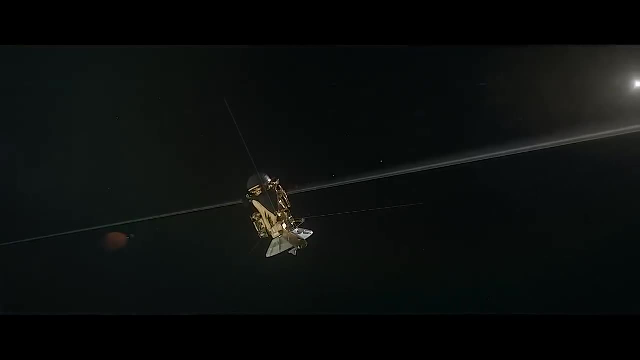 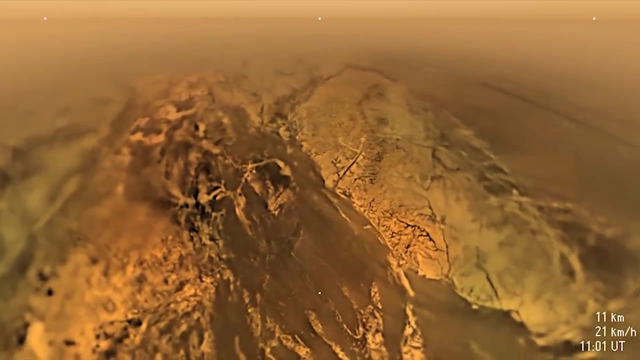 own mission one day. Cassini has done a great job, but it was never a Titan orbiter and its mission will soon be over anyway. What I would find extremely fascinating is to explore more of its surface, and hopefully it won't be long until a mission to do that will be approved.